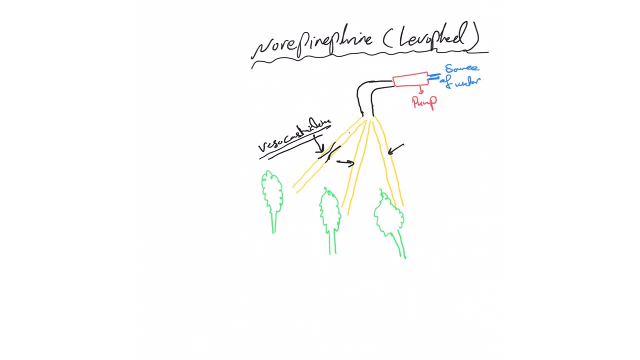 you can get if you have the same volume going through on a small diameter, that the pressure will increase. so that's the first thing also levophed or norepinephrine will cause. he will work here as well by increasing the strength of this pump as well as the frequency. so it's 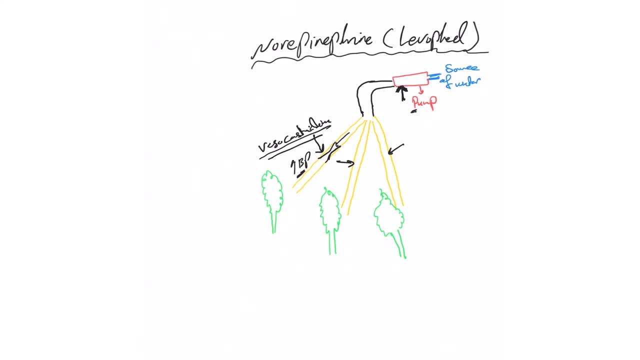 increase the pumping effect plus the frequency effect, so it has inotropic and chronotropic effects. that's how it works. but remember, with all vasopress- I'm going to keep saying this- you have to have the water, the source of water, if the patient is volume depleted. whatever you do, 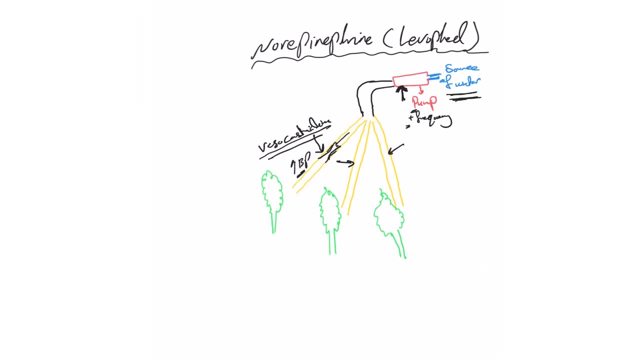 here if it's going to work. we're going to work temporarily and things will crash right after. you have to supply the water, you have to make sure the patient is adequately resuscitated with IV fluid and remember, if you don't have time to think, just give the patient two to three liters. 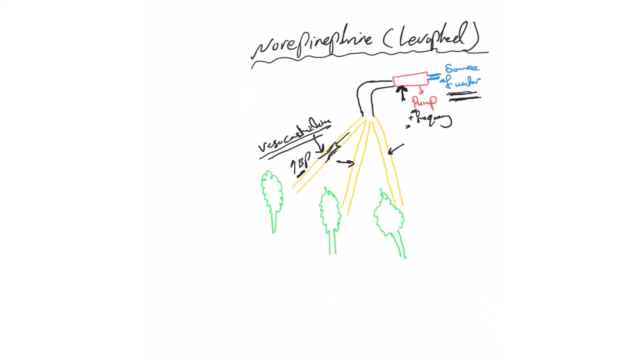 the only contraindication to give is pulmonary edema and you can give normal saline or lactate ringer, whatever, and you pick one of these two. there is no difference. so that's the first thing about how levophed works, and because of this, 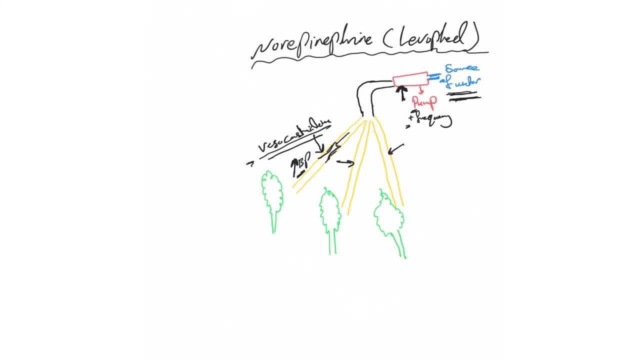 blood pressure increase right and the constriction, narrowing of the vessels- here we mentioned that it will increase the frequency but be in the body because of this constriction that will send a message to the pump and because of this till the pump to decrease the frequency again. all of this 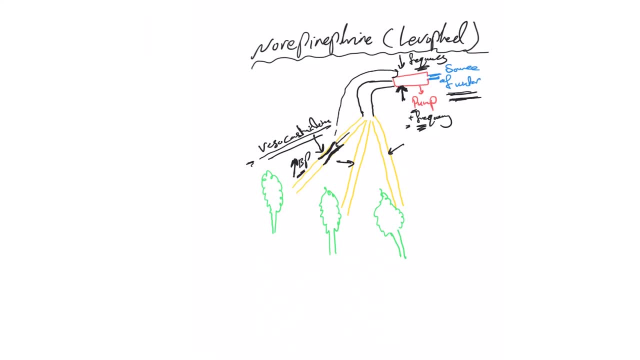 know in in physiology. I'm not going to try to explain why, but the vasoconstriction will send a message telling the pump to decrease frequency and the levophed direct effect telling the pump to increase frequency. these increase here and decrease here will cancel each other. so the outcome of levophed on heart rate is equal, so there is no tachycardia or there is actually mild bradycardia. so that's, if you somebody's on, you all the patient's tachycardia who should use different vasopressor till him know the effect of levophed or norepinephrine on the heart rate. is minimal. actually, it may decrease the heart rate. now, despite that, you may still. one of the side effects of levophed is arrhythmia. a quick with: leave what you have to give it through central line. now, if you don't have a central line, you can use peripheral lines for 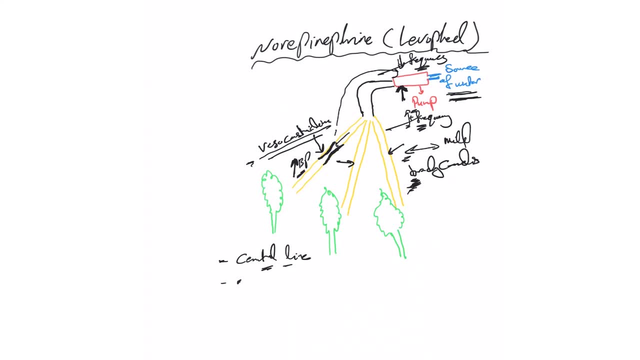 a few hours but you have to use a central line to avoid extra visualization. if the patient has levophed extra, visit into the tissue immediately DC it and give phentolamine directly subcutaneously into the tissue to induce vasodilation and prevent skin. 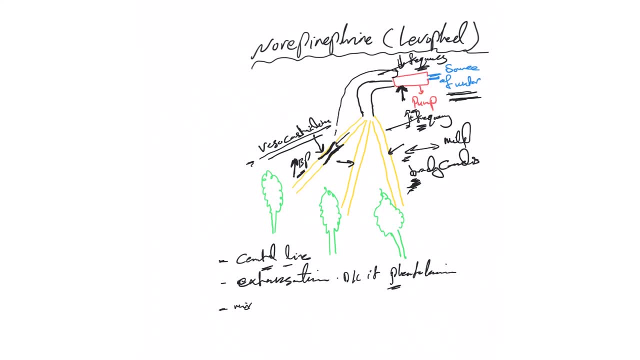 necrosis. usually it's mixed with d5w, some they mix it with normal saline. if you use too much vaso dosing- and again you can- I usually don't worry about dosing because pharmacist they can help us with that, but usually they start 8 to 10 mcg per minute. all vasopressor. we use mcg per minutes. 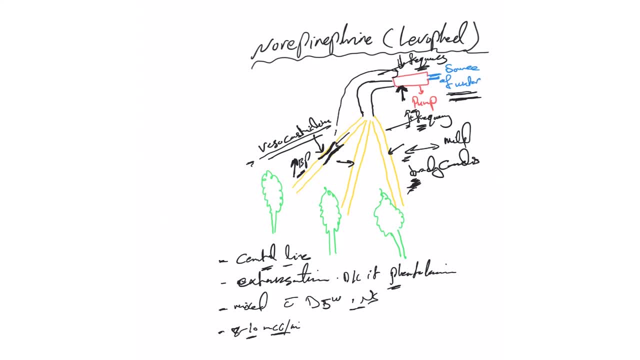 now, what's the maximum dose? nobody knows. some nurses say two mcg of some pharmacy per minute. I've seen 30 and 35. I've seen some intensive is using 50.. again, you want to avoid over or extreme vasoconstriction which can lead to dusky toes and fingers, because 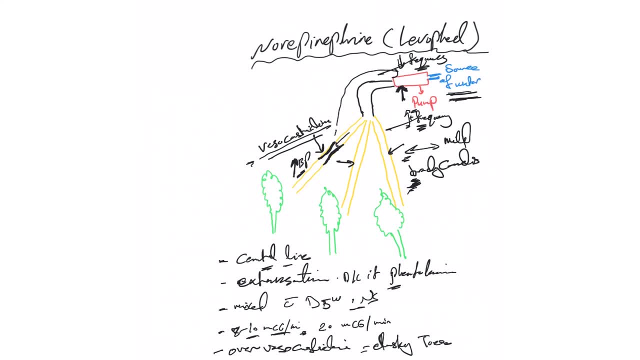 they cause severe vasoconstriction to these organs and may include oliguric aki. so, because of this, you want to make sure, using the minimum amount of levophed to maintain map above 65.. remember, with levophed it's the first agent to 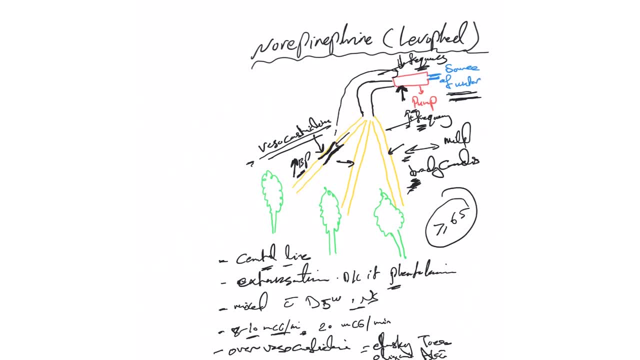 use whenever you're dealing with shock, except anaphylaxis where you use epinephrine. so if you want to think, just remember any case of shock, go ahead and use levophed, you will be right as long as it is not anaphylaxis. and remember not to forget about giving IV fluids. thanks, 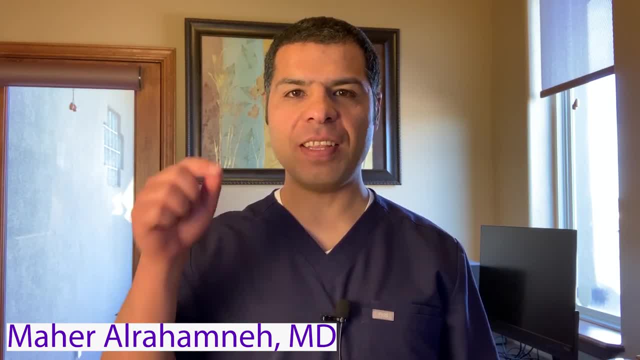 for watching this video. please subscribe to our channel and activate the notification Bell so you get to see the videos as soon as they are released. glad to have you on board.